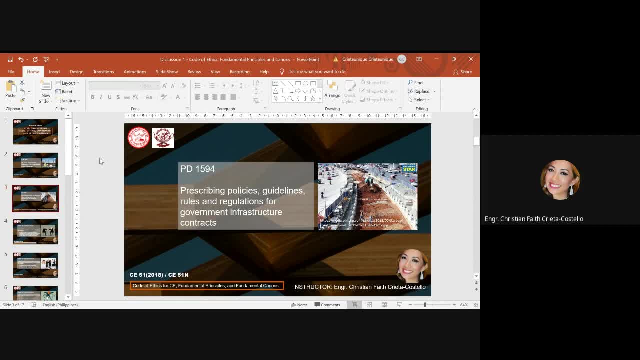 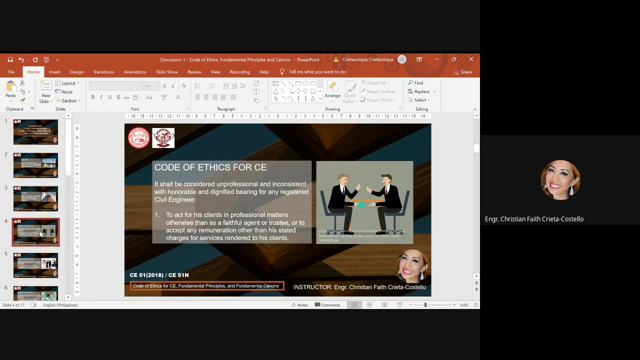 for government infrastructure contracts. However, we are going to dig deeper into each of the RA 544 and 1594. after we will be able to discuss the Code of Ethics for CE Fundamental Principles and Fundamental Conjunctions. Now let us start with the Code of Ethics. 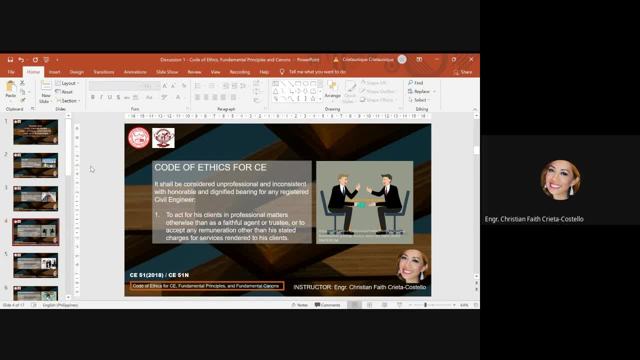 for CE or for Civil Engineers. It shall be considered unprofessional and inconsistent with the honorable and dignified bearing for any registered Civil Engineer if he or she is to act for his clients in professional matters otherwise than as a faithful agent or trustee, or to act for his clients in professional matters otherwise than as a faithful agent. 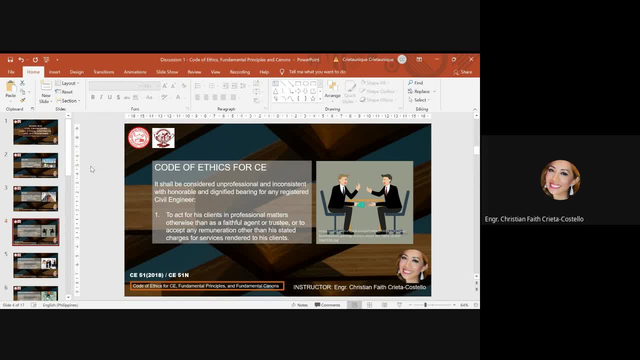 or trustee, or to act for his clients in professional matters otherwise than as a faithful agent or trustee, or to accept any remuneration other than his stated charges for services rendered to his clients. Maybe, upon reading on this Number 1 Code of Ethics for CE, you 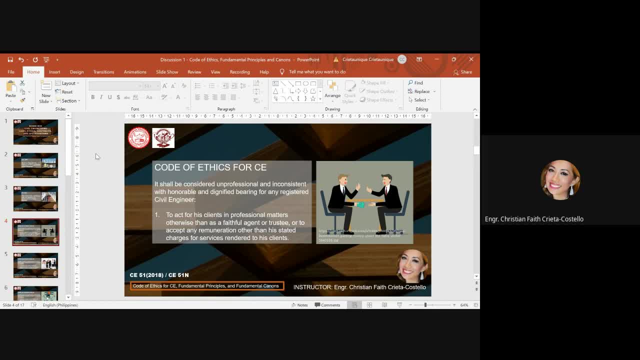 will literally have in mind what is commonly referred to as under the table payments or if clients, if some clients would want to have a faster processing of their documents and there could be a point where in you will offer you extra money aside from your usual rates for remuneration, so that you will prioritize. 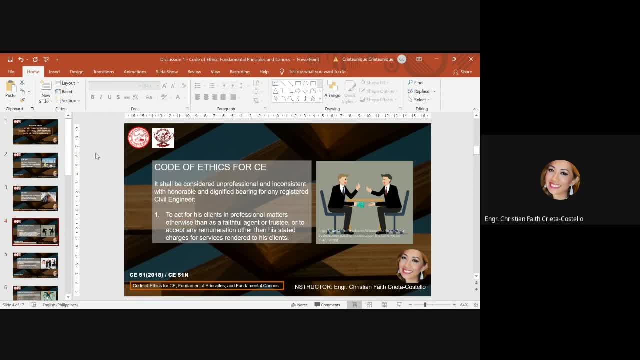 their documents. however, under the code of ethics, you should not be accepting or you should not be tolerating any of this act, since it is against the ethics of civil engineer. it would be unprofessional for us to do that. next is still: it is unprofessional for us. 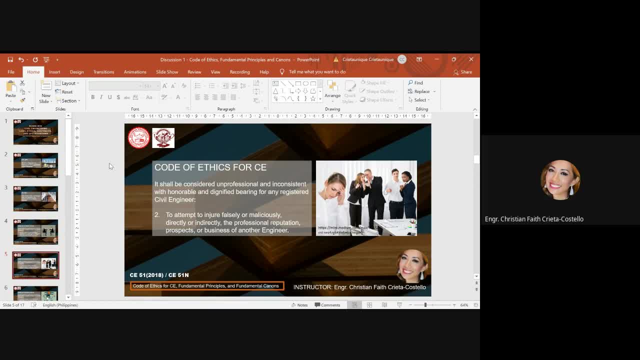 to attempt or ensure falsely or maliciously, directly or indirectly, the professional reputation, prospects or business of another engineer. mainly, this could be rooted to what we call as jealousy in work or in the business. however, as an ethical engineer or civil engineer, you should not be doing any negative or any. 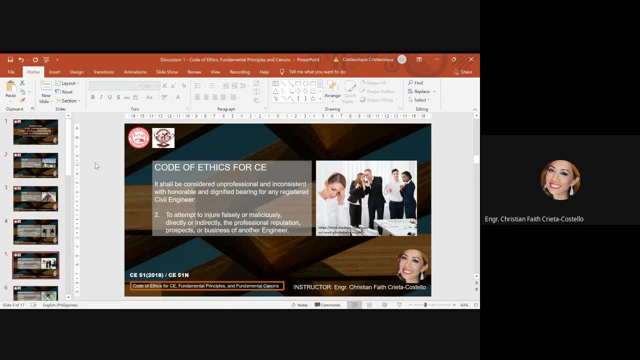 bad things, bad things against your fellow civil engineers or fellow professional just to make you look good. it is very common, especially if you will be working in the real world as an engineer, as a civil engineer, wherein other colleagues might get jealous of you, especially if you are doing good in your work. so some of your colleagues 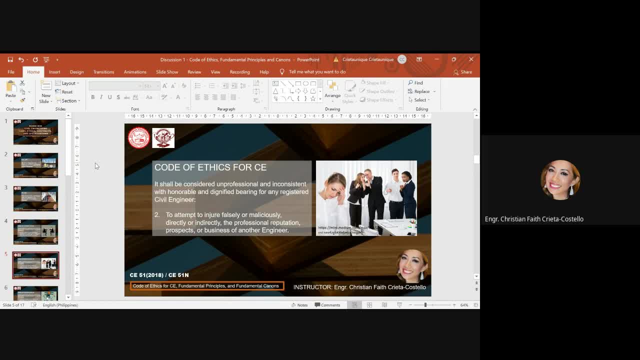 who are jealous to you, might be pulling you down and will be making up stories that could make you look bad to your employer. in order for you to avoid situations like this, just keep focus on what you are doing and never entertain and, at the same time, never do this kind of thing against your fellow engineer or your 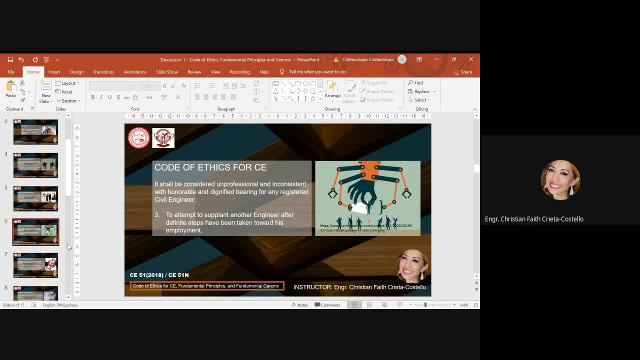 co-workers. next is: it is still unprofessional for us as a civil engineer, to attempt to supplant another engineer after definite steps have been taken toward his employment. so samples: and for this is if you are both working together for a higher level position in your employment and then your fellow engineer or your fellow co-worker had 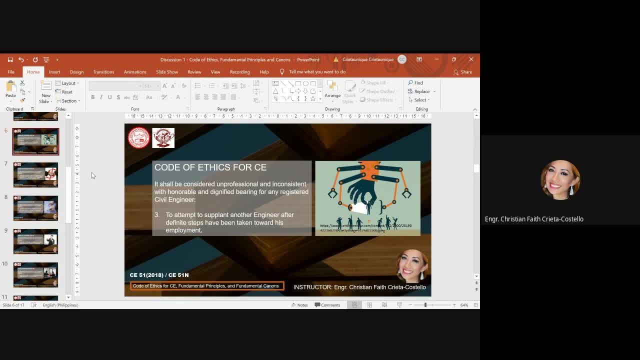 done steps ahead of you in good will. however, since you also want to be ahead of him or her, then you sorted on doing something bad which can make your work ahead of him or her. then it is very unethical for you to do that. let us think, for example, for direct situation, and this say, for example: if 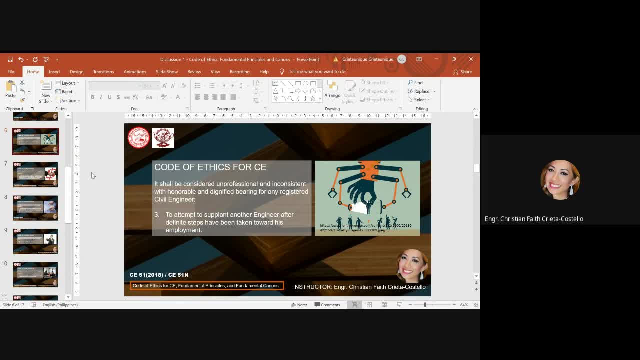 even as a student. we can make a sample situation for this one. say if the teacher is giving you an activity and then you are a bit lazy to start ahead on the activity. however, some of your classmates had been starting already doing the activity, but since you want to compete with them, trying to look 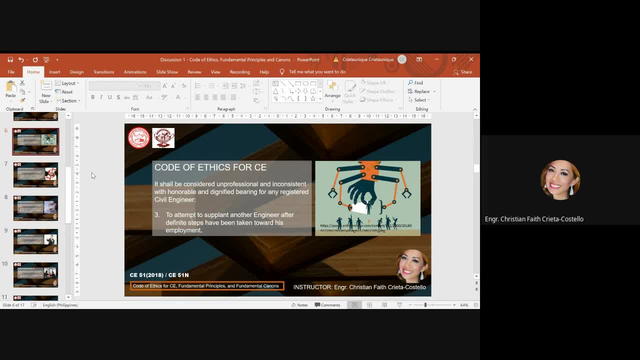 good to your teacher, then you simply copy what your classmates are doing. then it is too bad and too unethical for you to do that. therefore, as a students, as a start, make sure to avoid behaviors like that so that you won't be able to bring it in the real world when you will be working as a civil engineer soon. next is 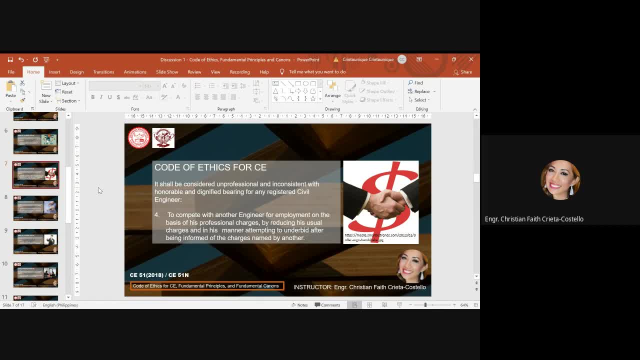 still, it will be unprofessional and unethical for us, as a civil engineer, to compete with another engineer for employment and the basis of his professional charges by reducing the amount of work that he has to do and increasing his usual charges and, in his manner, attempting to underbid after. 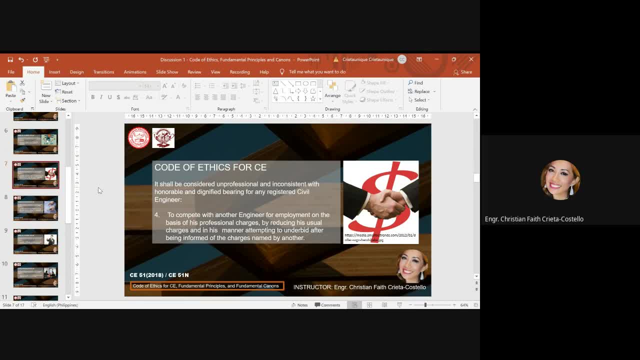 being informed of the charges named by. another example situation on this one is say, if you own a company and also other companies are included in the bidding wherein you join. however, however, since you wanted to win in that certain bidding of construction project, then you try to give money to the officiating officials, to which other 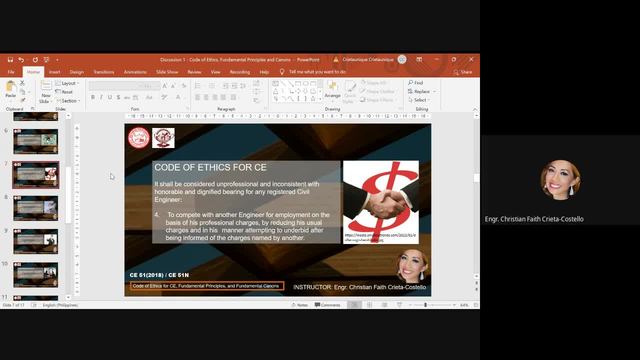 bidders of course doesn't have any knowledge of, then it is very unethical for you to do that. also, sometimes there are some construction firm wherein they tried to befriend the bidding officials and it will end up the bidding official giving them informations for all the prices of. 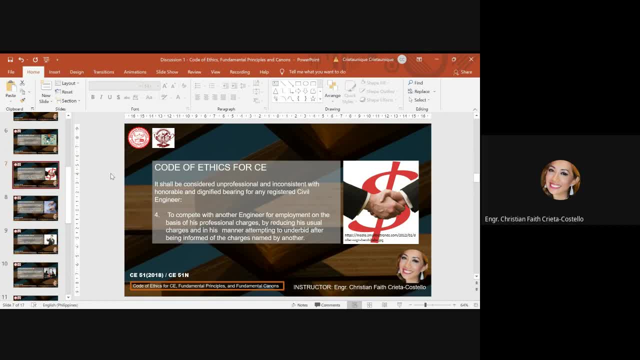 other bidders. therefore, this is already a big mistake, because most of these businesses, if they even have a bid AMPLIFE, they can already adjust their submitted price and make it or try to lower it down so that they will be the one to win in the bidding. by doing things like this, then, you are no longer doing a fair play, which means very unprofessional, since. you got to be a fair play to win the bidding. so when you are doing something like this, then you can no longer win in the bid by doing something like this personally, or you can do it online, if you choose to do it online. so there is no problem with that. 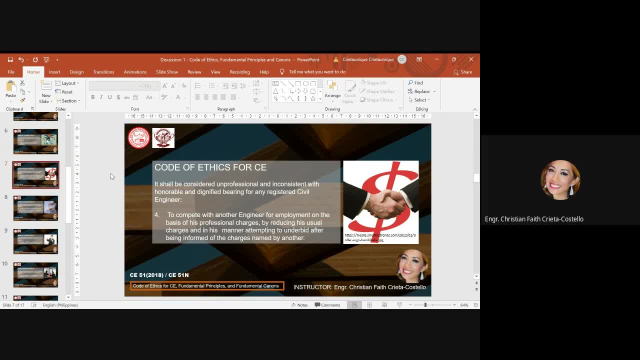 considering the word bidding, you should do it fairly with other bidders. you should always be careful, even if you're just an employee or even an owner of your own construction firm. try to avoid things like this. next, still, it is unprofessional and unethical for us to review the work of another. 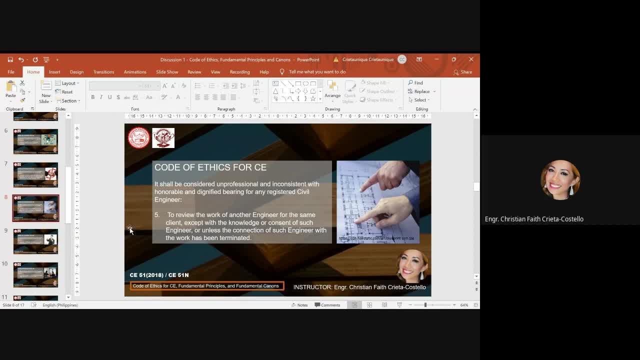 engineer for the same client, except with the knowledge or consent of such engineer or unless the connection of such engineer with the work has been terminated. when this number five was discussed, there is a question that has been raised that why can't we review the work of other engineers, since it would just be for the purpose of trying to make sure that his 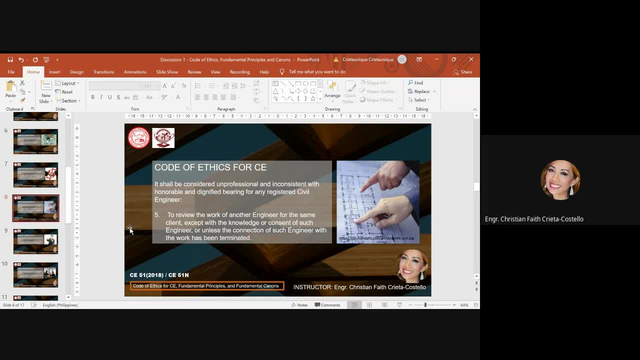 work is okay. however, it is very clear here that, except with the knowledge or consent of such engineer, or unless the connection of such engineer with the work has been terminated, or unless, if you are considering an employee of a certain company, do not ever try to review the work of your colleague if you are. 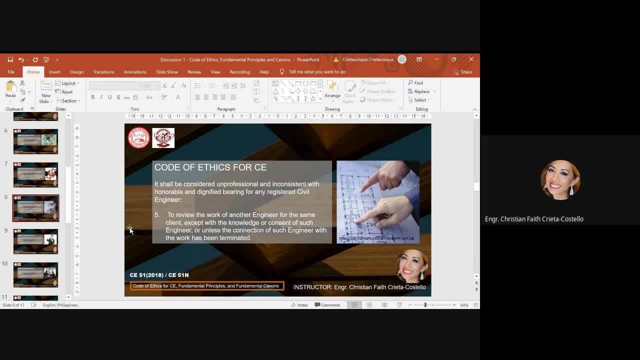 not asked by your employer, since it will create issue with your colleague who is doing the work. if your employer did not ask you anything to review his or her work, then do not do anything about the work, since it will just make your colleague look like making mistakes or cannot be trusted. also, if you are going to attempt to, 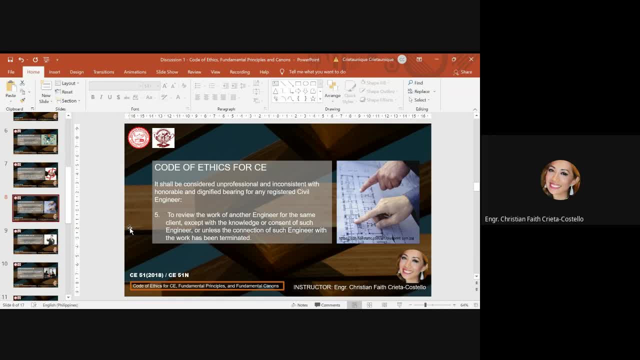 do or to review the work of another engineer, then it means that you are always just suspecting that his work is not good enough, and having this kind of mindset is very unethical, since, considering that he is already an engineer, that you should have trusted his skills and 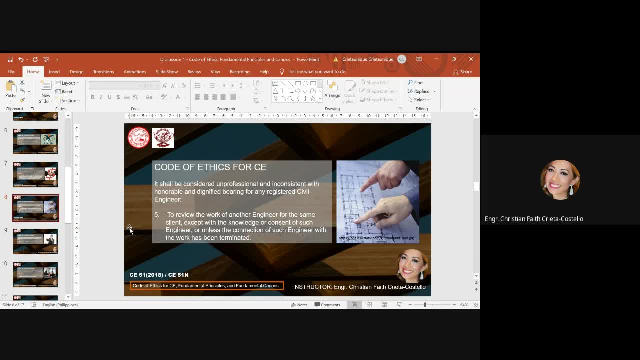 abilities because he already got to what work, where he is already like he became an engineer. trust him as an engineer. unless it would be your job to review their work, then you can do that, but if not, then never do that. next is still. it is unprofessional and ethical for us as a civil. 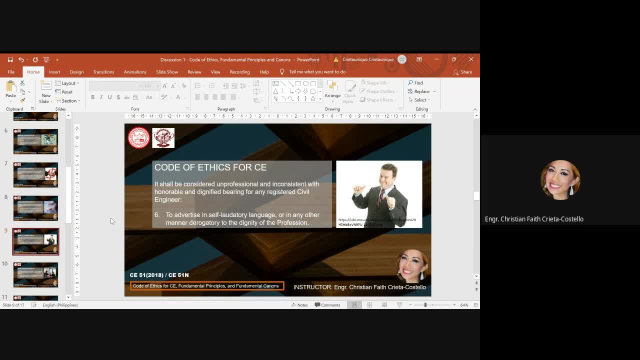 engineer to advertise in so floutatory language or in any other manner derogatory with a dignity of the profession. so meaning self-laudatory language, advertising self-laudatory language. it means even if you're already a civil engineer someday, just try to be humble and not to be boastful. 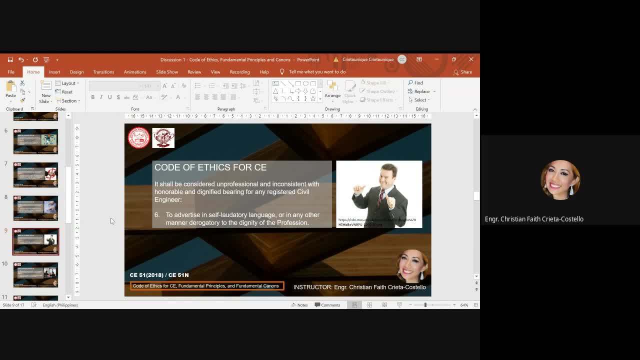 um, anyway, um, your profession and your work ethics will say more rather than what you will be talking. and then do not also do any derogatory things that could affect the dignity of our profession as a civil engineer. there could be a lot things that can bring negative effect to our profession. this is to avoid. 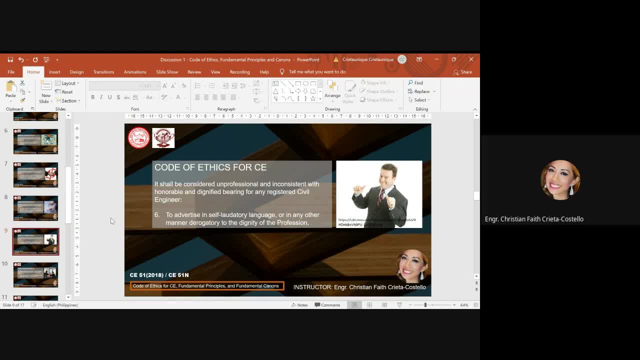 us or from being from like. if you will be doing such things, then there could be a possibility- possibility where our license as a civil engineer could be revoked. so always try to be ethical and professional, whether you are in work or outside work, because you are now um trusted or you are now holding um an honor related to the profession that 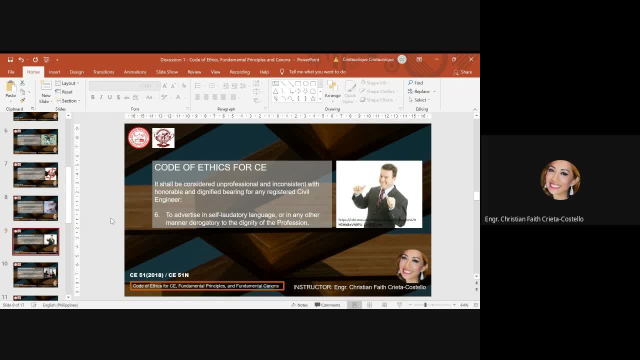 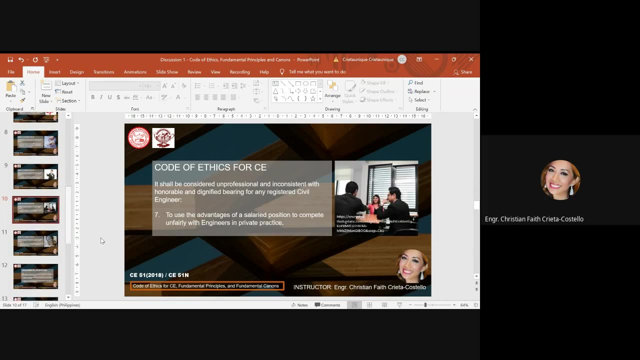 you are working hard for how many years in college and um, after the licensure period exam? now we will talk about the number seven, which is still. it is unprofessional and unethical to use the advantages of a salaried position to compete unfairly with engineers in private practice. advantages of a 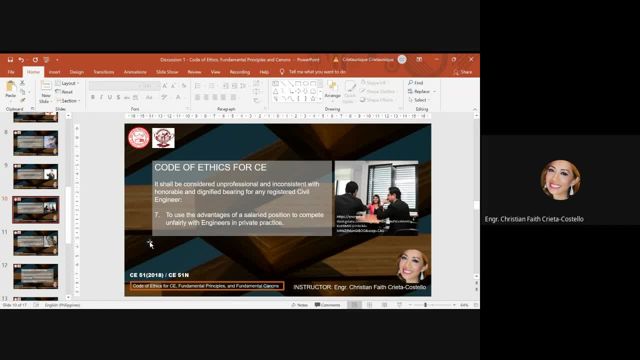 salaried position to compete unfairly with engineers in private practice. okay, sample to this one is: if you are, you are working or competing to get a certain project. however, you are an engineer of a government office and then your competitor is an engineer of private company and since you really want to get that project, then you try to use all 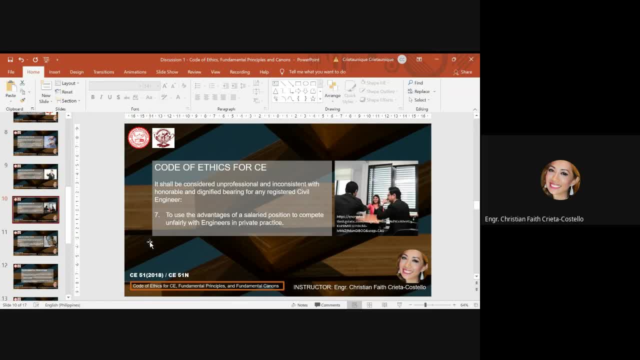 your connections in the government so that the that project will be given to you. so of course with the representative in the private company. since they are only a private company and considering that they are still a small company, then they have less connections, then they cannot surely win the project by doing this. it means it is very unethical and unprofessional. 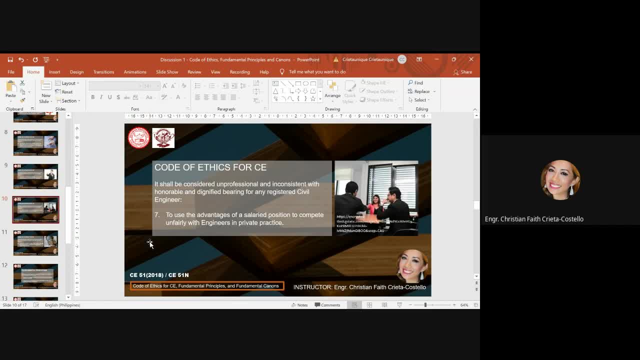 to also. we can give also a situation wherein civil engineering students will be sent under OGT or under housing and since this, under job training, civil engineering students will be at some point working together with civil engineer education that will otherwise be sent under and your training will appear because you mainly mostly, are under". 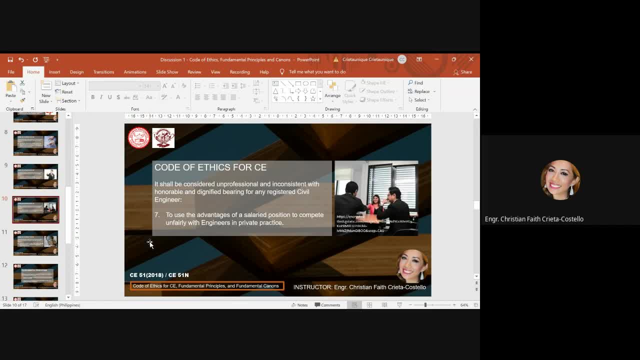 level in nationale. also, we need to be method behind. education does not but veryシ coping specifically private student smalllı, while alsoisk the with already professional civil engineers. I've heard stories where in professional civil engineers are behaving like arrogant and trying to like look down on the OGT students and they tried to make the OGT students 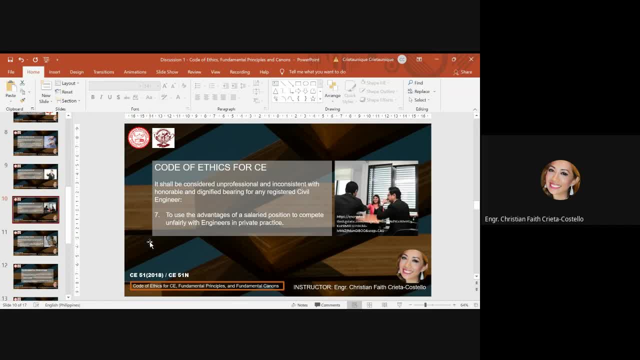 feel very small, instead of giving them training on how to feel like being a civil engineer. so doing things like this is also considered unethical and unprofessional, so never always take advantage of your position to unfairly deal with other engineers or even other co-workers in a certain company. now, still, it is unprofessional and unethical. 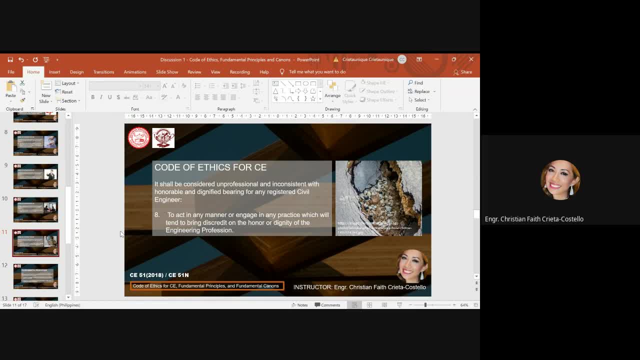 if a civil engineer will act in any matter or engage in any practice which will tend to bring discredit on the honor or dignity of the engineering position. in the sample picture I am showing to you some substandard road. it is commonly happening in our country where in some countries if you have a civil engineer position you always have to reflect to them. where in some countries in our country, where in some 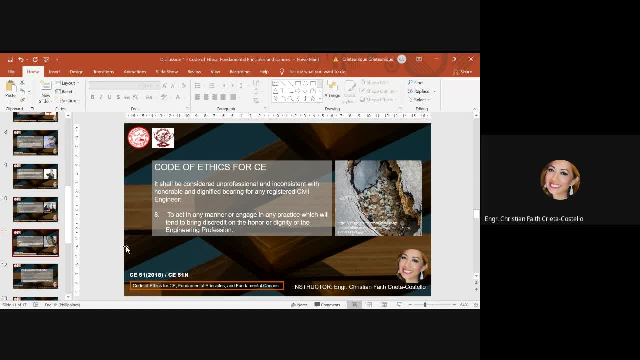 contractors are not really following the standard materials suggested to be used in certain road projects. maybe this is for them to gain more profit from a certain project, or they do not know what would be the underlying reasons why they are doing this. however, engaging into this kind of 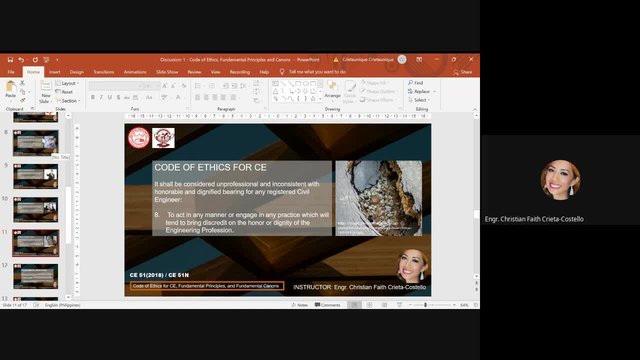 act is already considered as bringing discredit and honor to our profession in the civil engineering industry. so, as much as possible, try to um do good ethics, good work, ethics related to your work and related to your colleagues, and try to avoid any shortcut and try to avoid any. 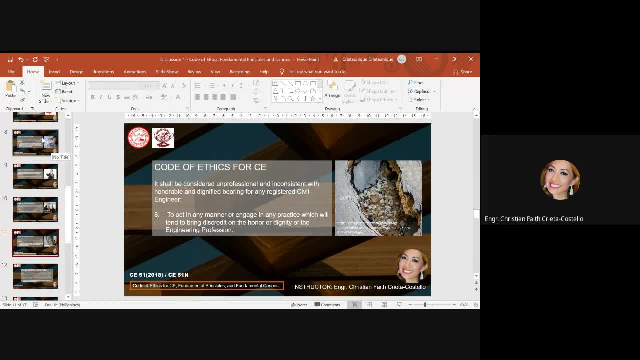 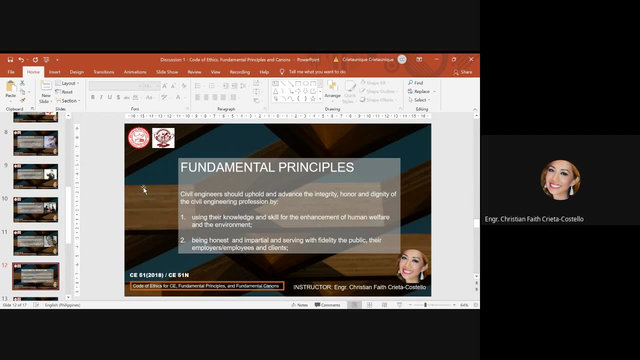 situation that could bring a negative impact to our profession as a civil engineer. now let us go to the fundamental principles. civil engineers should uphold and advance the integrity, honor and dignity of the civil engineering profession by number one, using their knowledge and skill for the enhancement of human welfare and environment. here we have to. 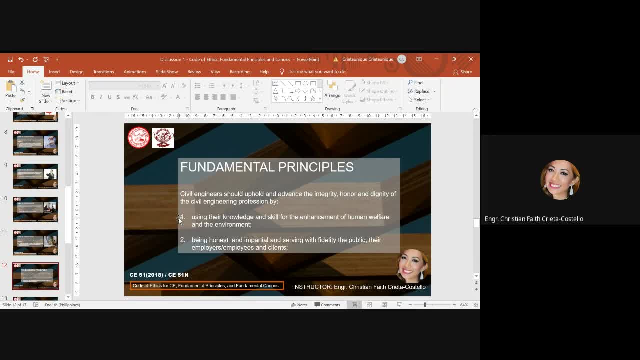 look at some of the basic principles of civil engineering. we have to consider, or we have to know, that we are not only getting our profession as a civil engineer simply to build and build and build, but we have to design and build something for the purpose of enhancing the human welfare and the environment. right now, it is a 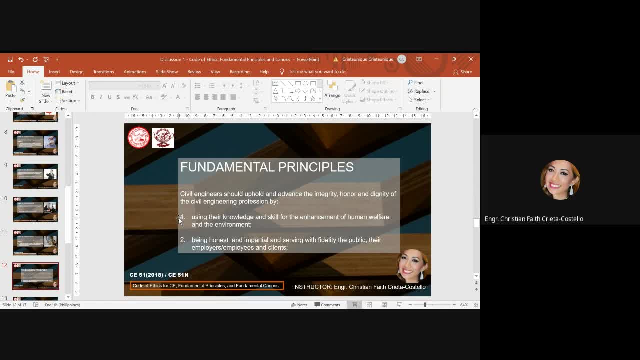 very well-known issue in um dumaguete: the 174 hectare reclamation or the smart city proposed by the, the officials of dumaguete. there could be two sides of the issue, the pros and the cons, and those who say yes and those who say no of the project. but in my own opinion, as a civil engineer, 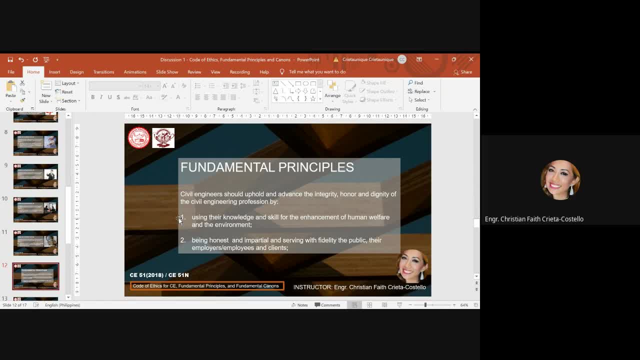 even if at some point it shows the development of the city for the island, but it also clearly shows a negative impact on the environment, then i am against project. so in this simple example, there is no longer consideration on the enhancement of the environment in regards to this kind of project. 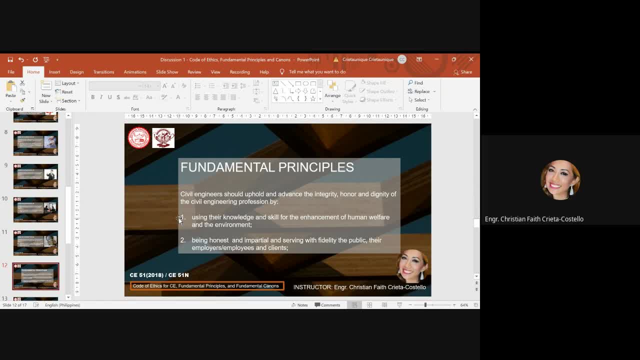 therefore, as a civil engineer or as a professional, you should also think that the project that you are doing is not giving negative impact to the environment, to the human welfare or even to the animal welfare. you should always consider the. you should always consider the good impact for everybody. number two: being honest and impartial and serving 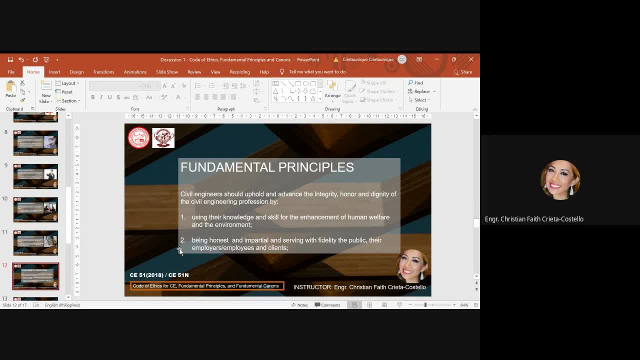 with fidelity the public, their employers, employees and clients. of course, we should always uphold and advance the integrity, honor and dignity of being honest, and so the transparency and complete honesty. next is number three: we should always uphold and striving to increase the competence and prestige of competence and prestige of civil engineering profession. 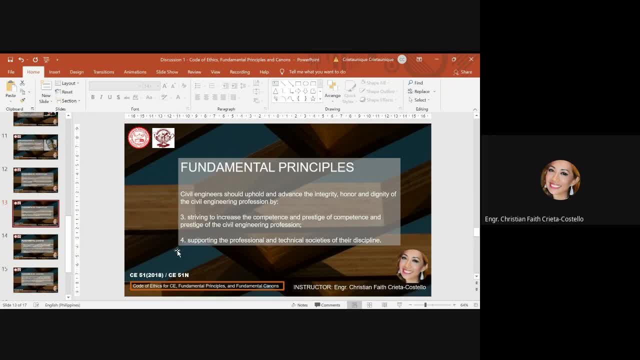 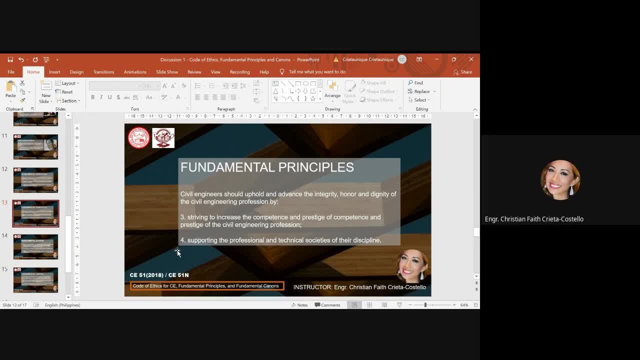 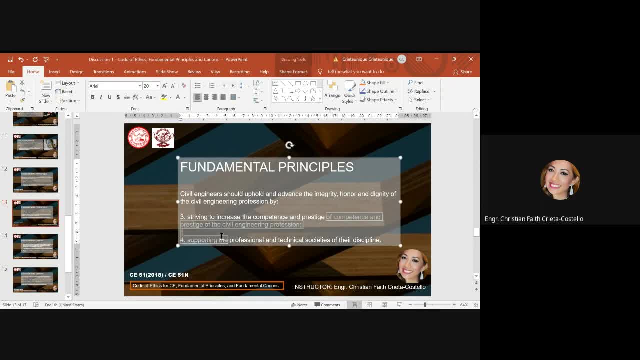 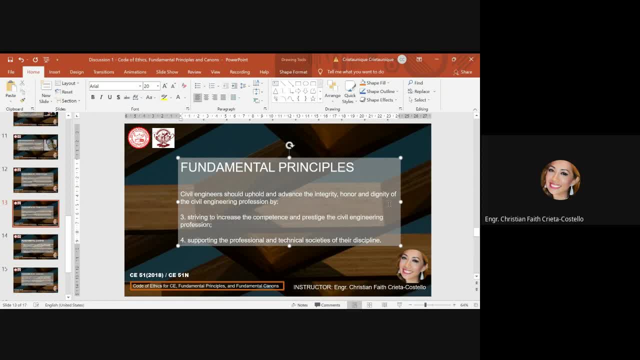 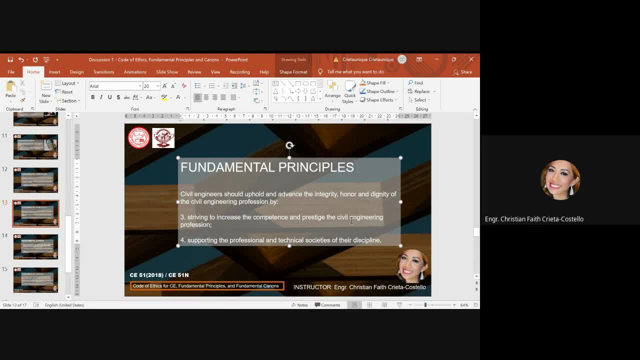 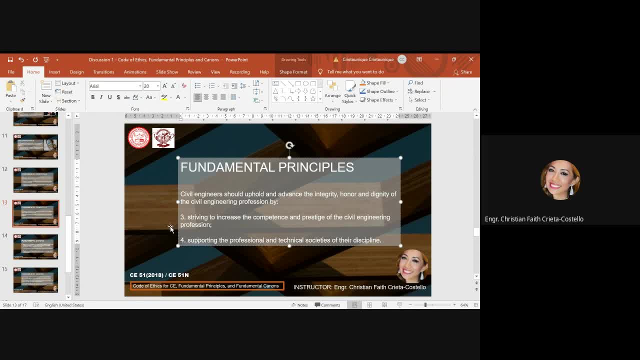 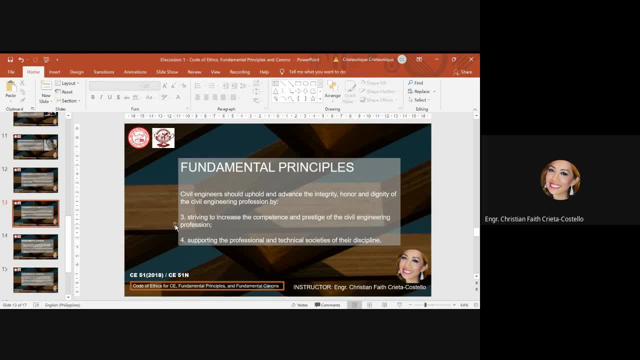 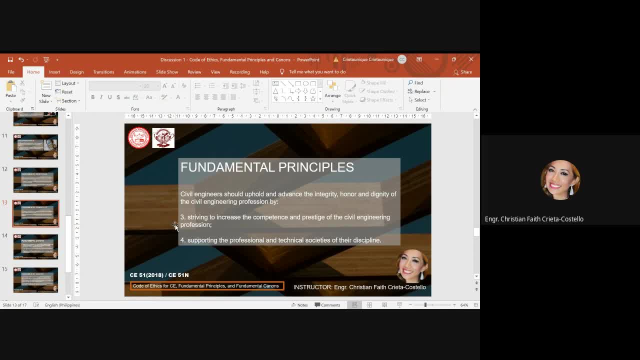 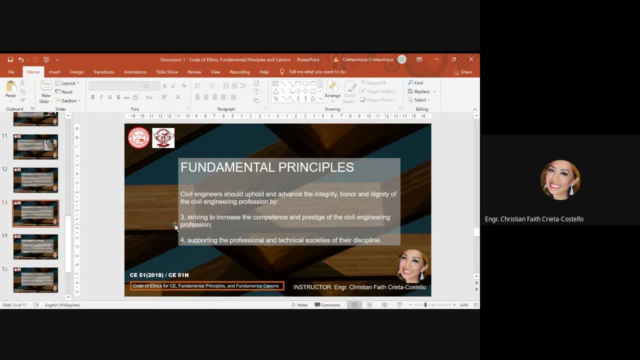 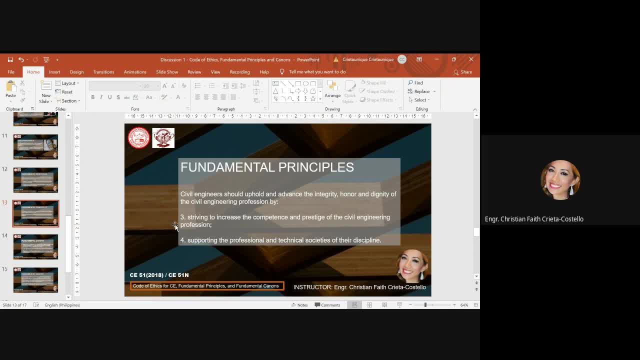 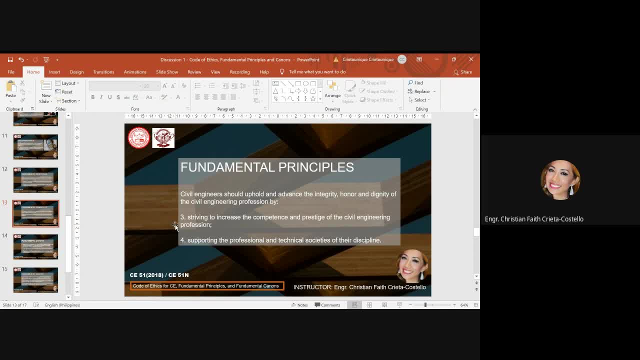 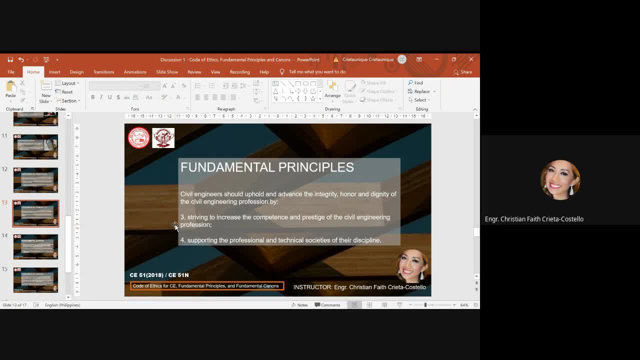 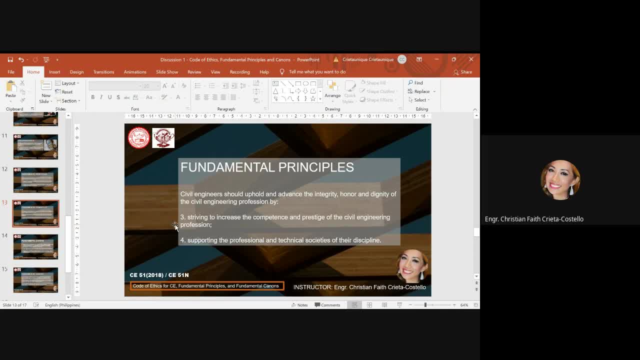 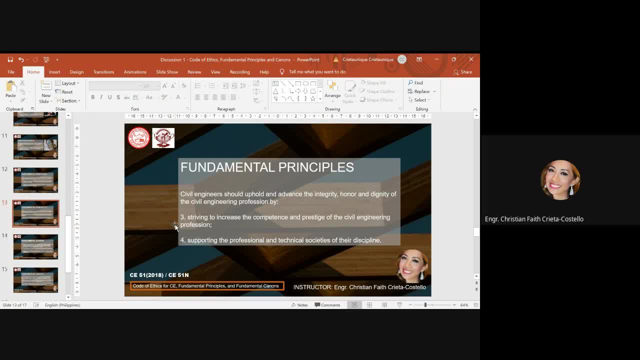 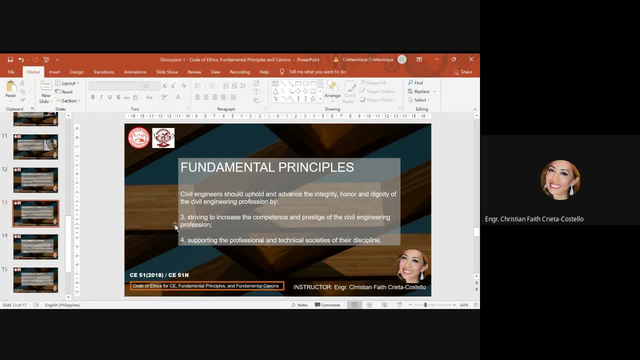 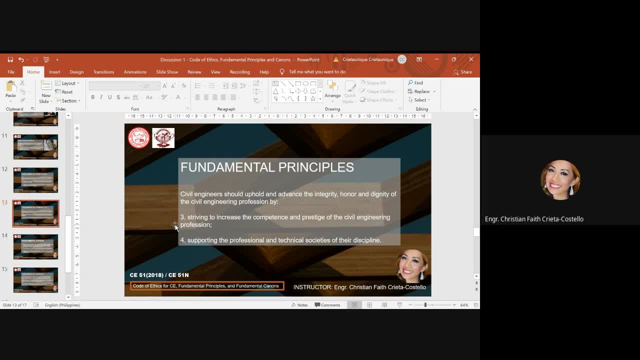 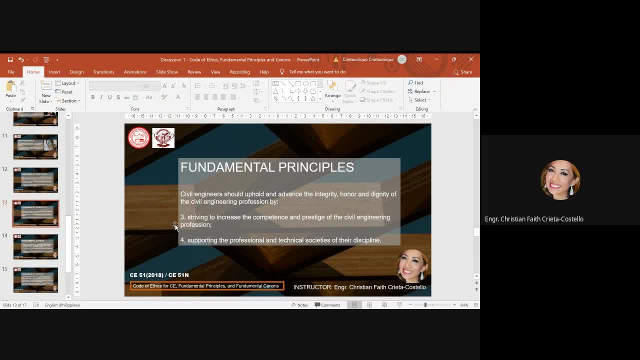 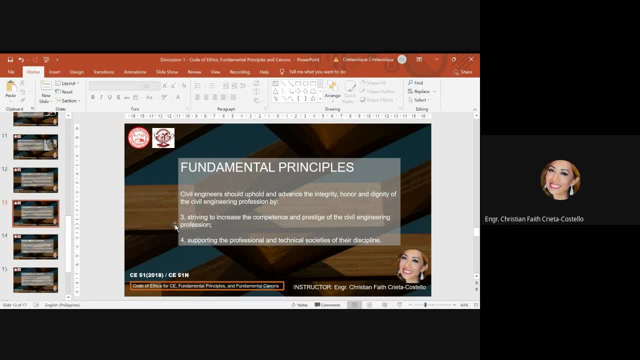 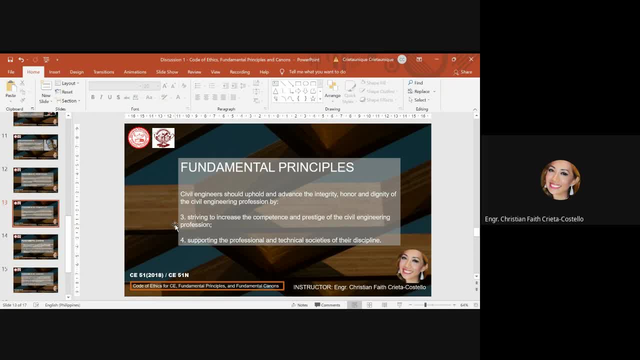 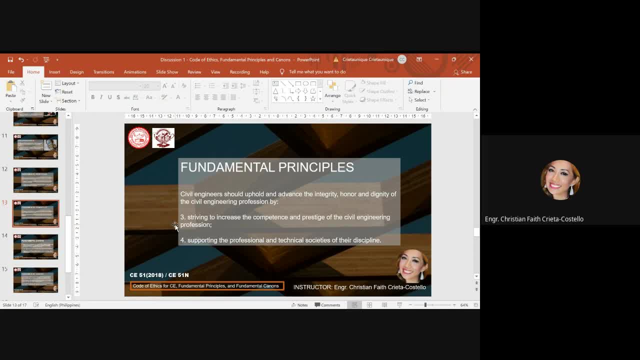 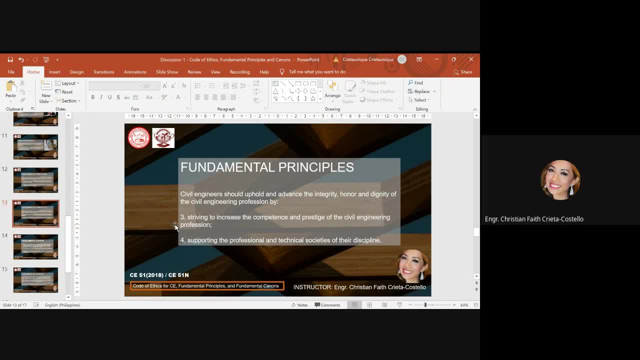 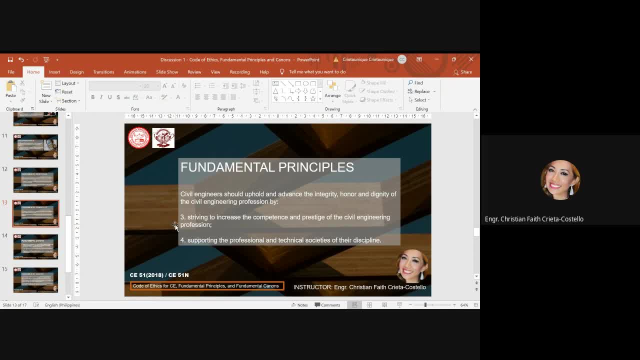 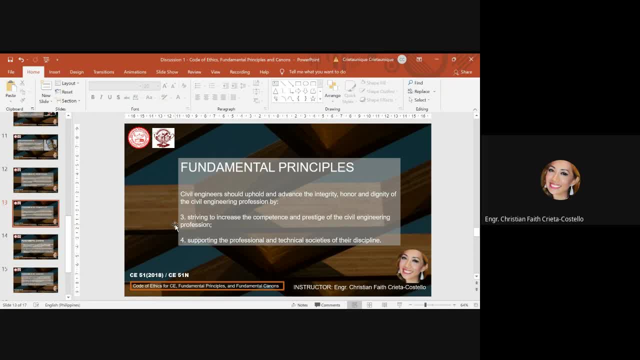 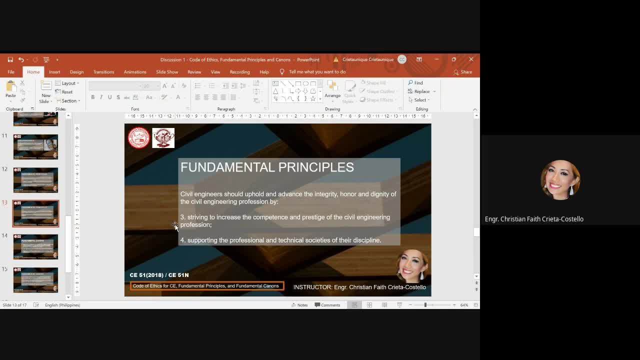 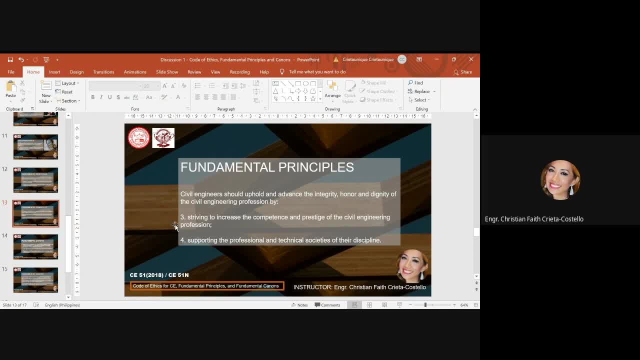 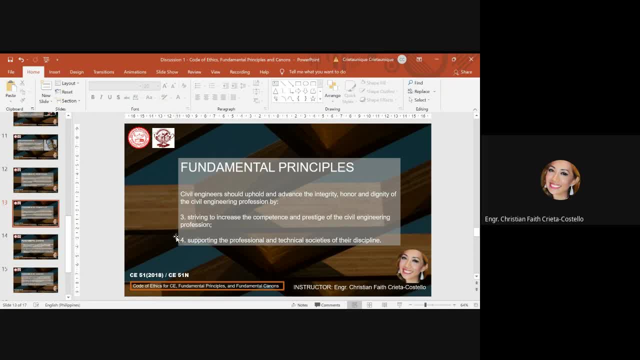 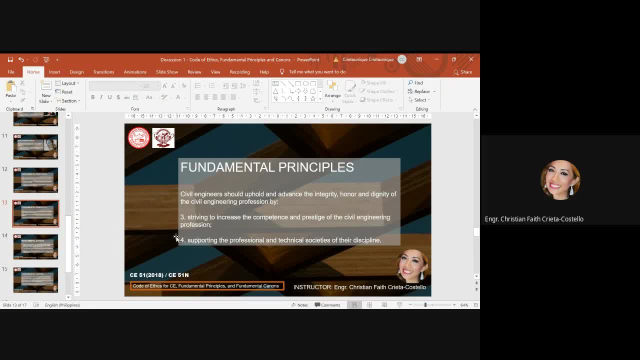 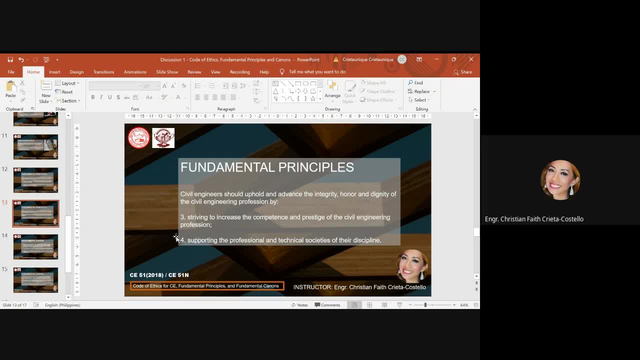 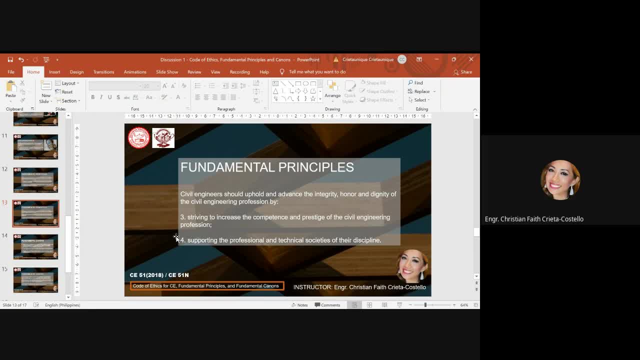 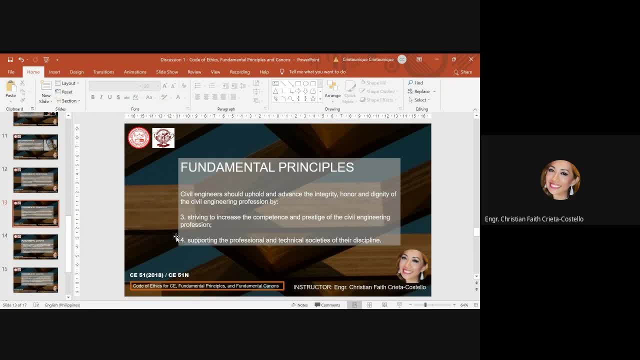 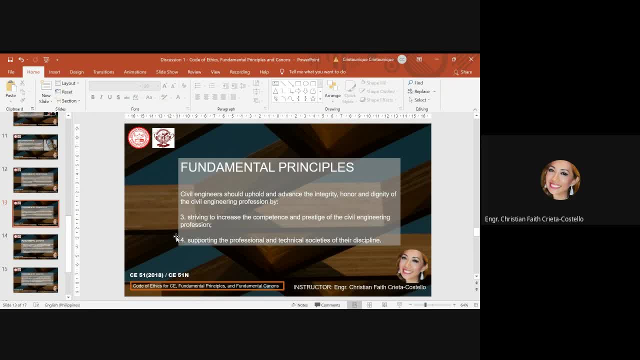 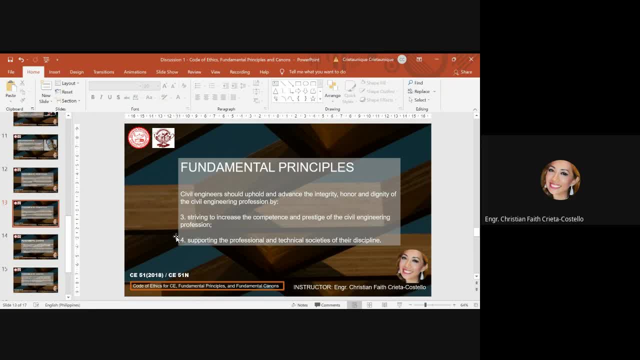 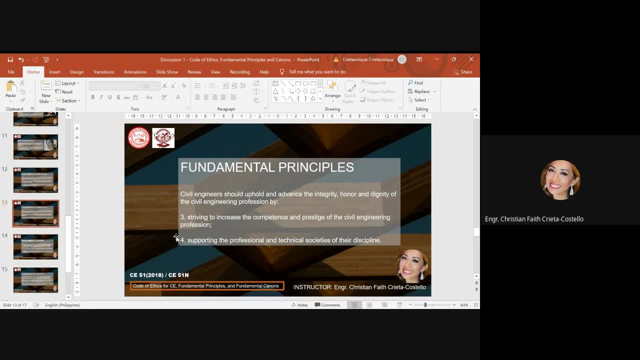 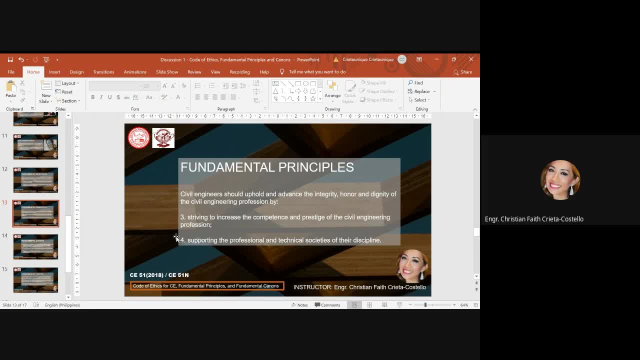 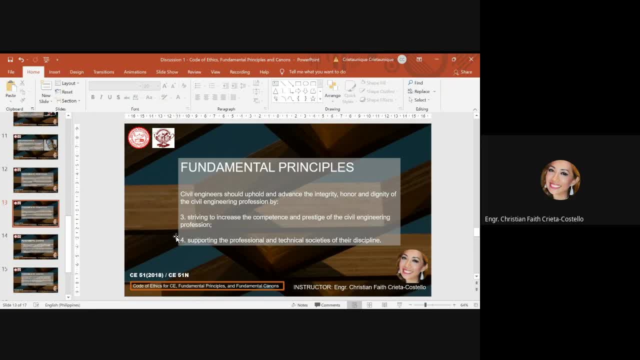 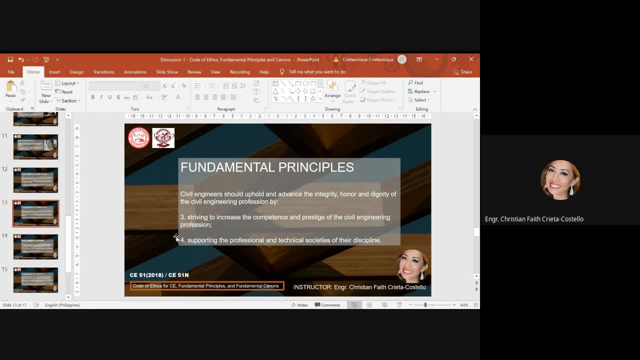 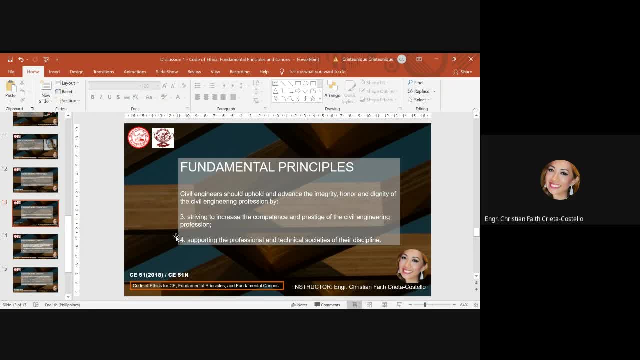 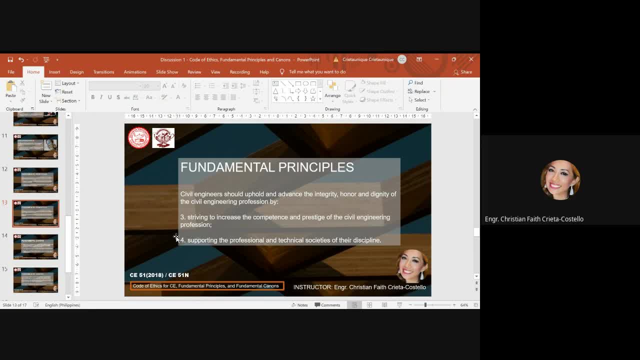 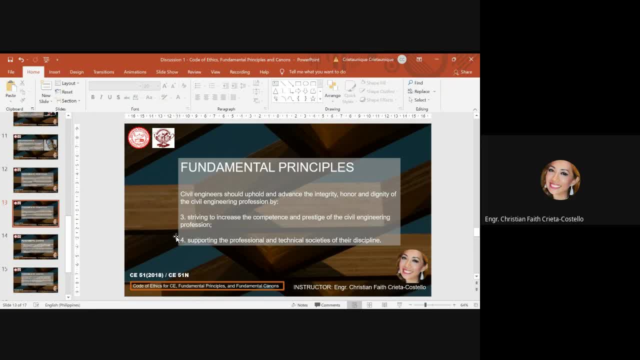 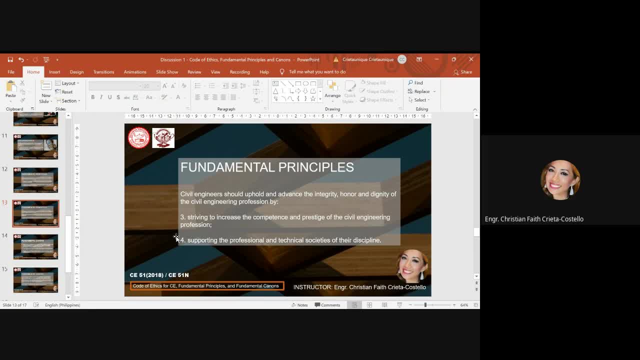 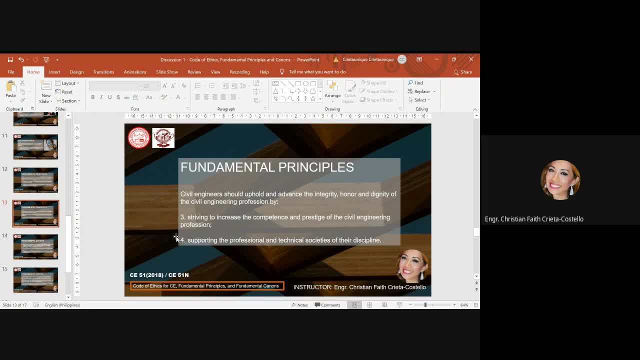 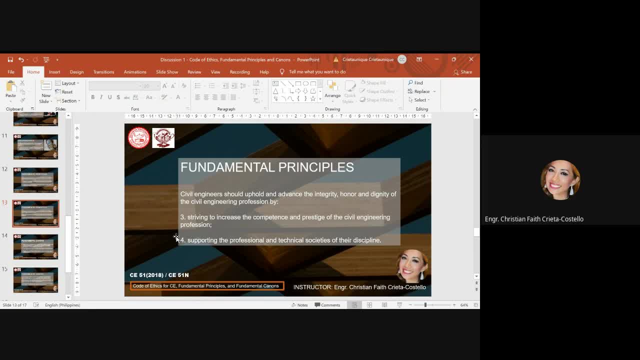 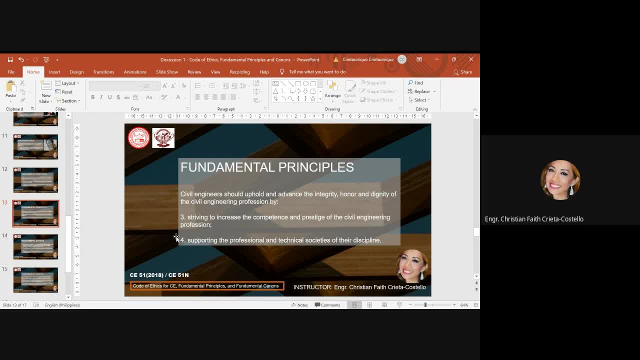 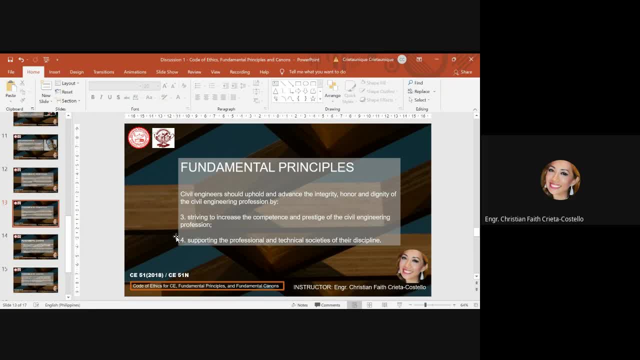 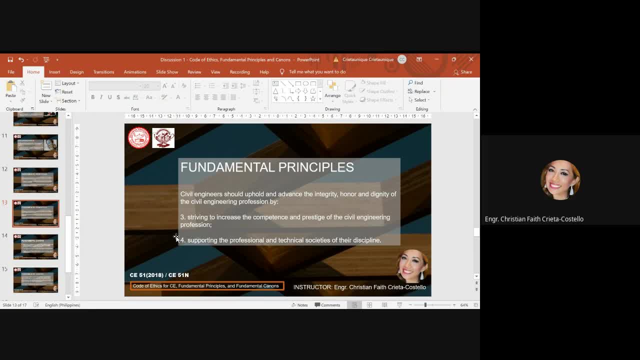 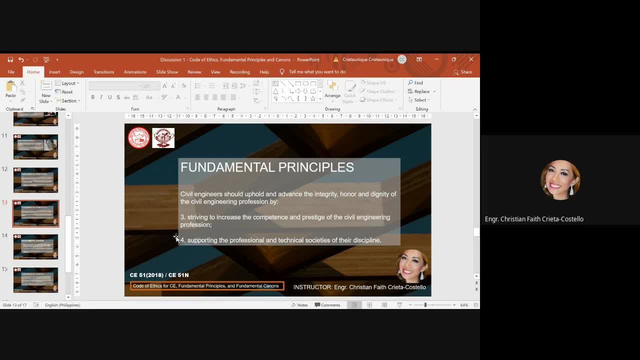 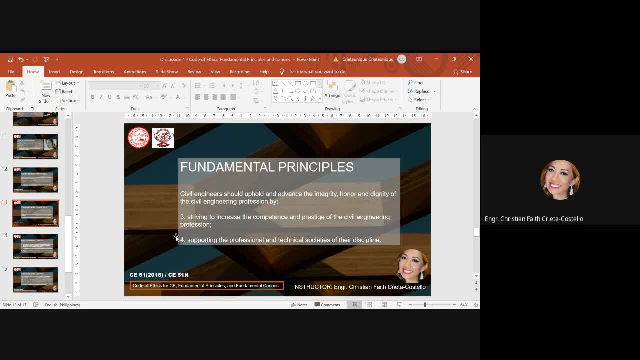 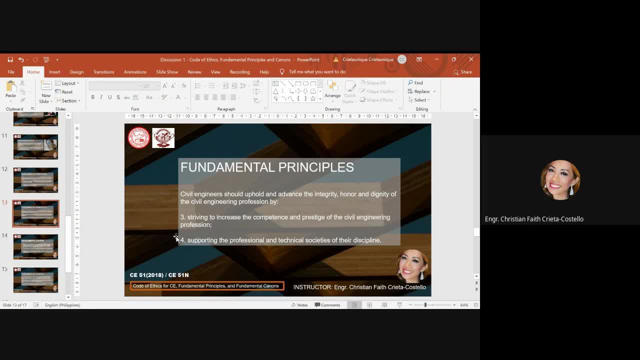 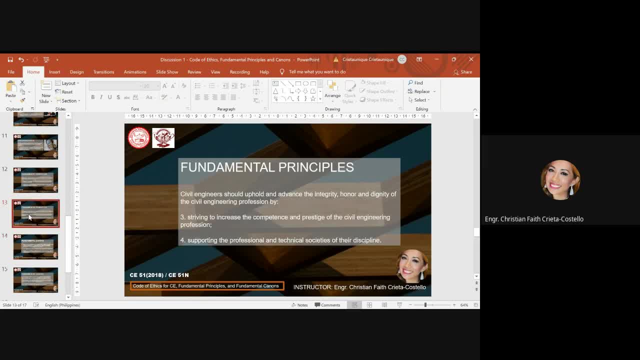 and prestige of civil engineering profession and prestige of civil engineering profession. Now we will go to the fundamental columns. Number 1. Civil engineers shall hold paramount the safety, health and welfare of the public and shall strive to comply with the principles of sustainable development. 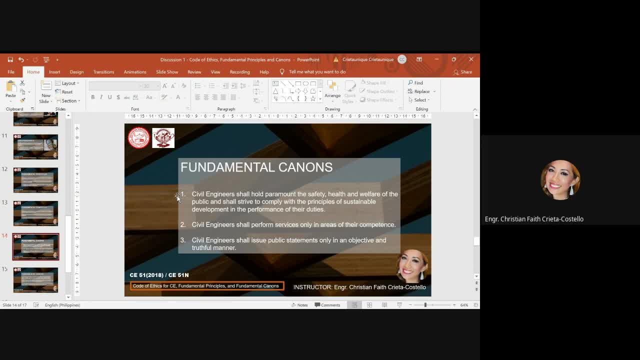 in the performance of the duties. So, as what I have said earlier, we should not only build and build and build without considering the safety, health and welfare of the public and the environment. It is our job to make sure that the project that we will be working should always consider. 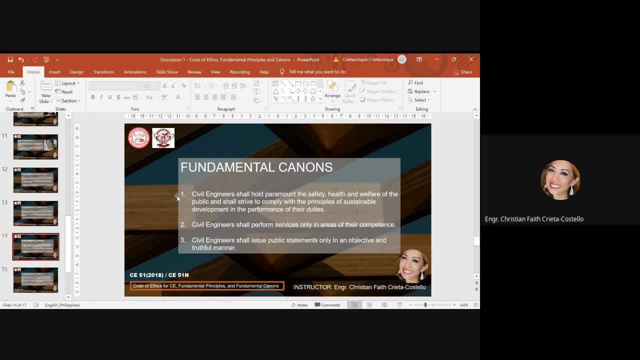 the welfare of everybody. Next is civil engineers shall perform services only in areas of their competence. This means that, as a civil engineer, you should only work in projects wherein you are confident of or you are advised to work with. And at some point, some civil engineers confused on. 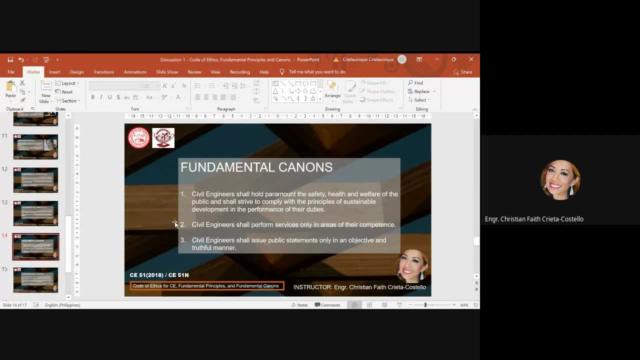 doing. what should they do? Good work for architects. i mean, some civil engineers are already doing work of architects, so this thing should be limited, because if we will be doing things that should be done by architects, then we are already getting or making their profession like non-existent. and also, even if you 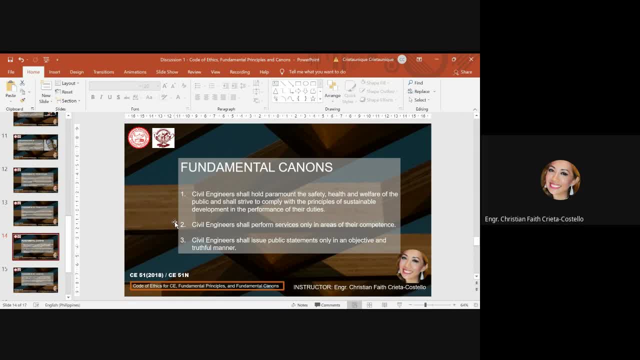 are a civil engineer already. it is undeniable that there could be some work related to civil engineering wherein you are not confident. of then, if your employer will ask you: are you confident to do this project- and in yourself you are not, but since you wanted to impress your employer, then you will say yes, i am confident- then it is unethical for you to do that. 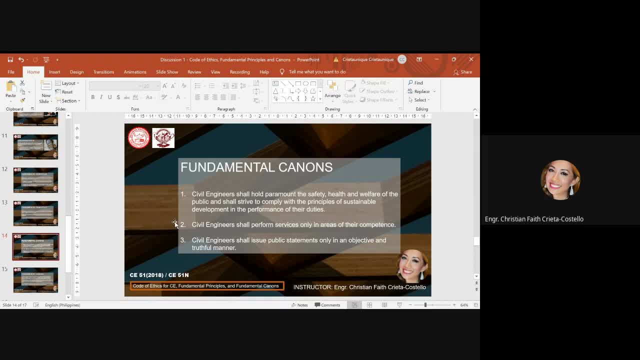 just be honest, like saying i'm not confident to do that project, but i am willing to undergo training. if you want me to assign on that project, then that could be a better way to communicate with your employer. next is civil engineers shall issue public statements only in an objective and thoughtful manner. there could be a point wherein you will be. 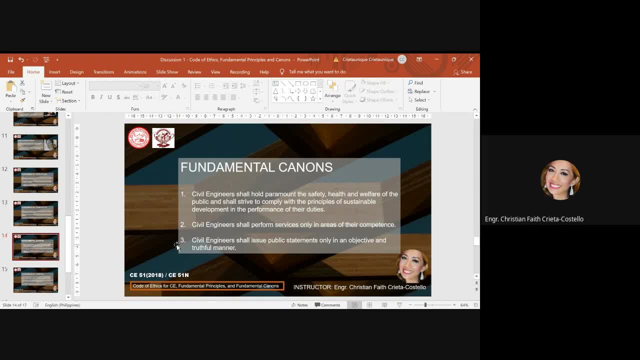 asked to issue public statements, especially if maybe your project involves in a failure, or maybe your project is involved in a huge like issue wherein you need to show or you need to inform the public of what is really going on, then what you have to do is make your statement in an objective and truthful manner. do not add or do not. 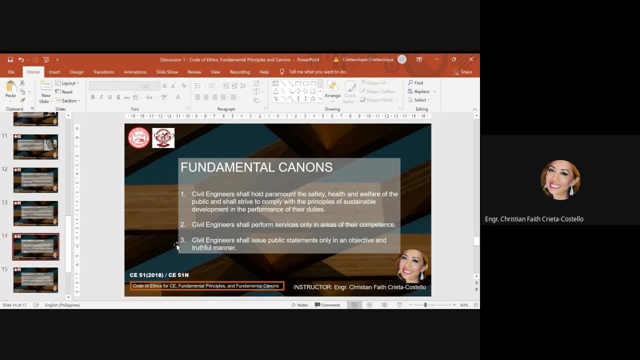 quote less details. however, make sure to give the exact information about what you should let the public know, like make as concise but complete details so that the public will really know of what is really going on. never add or never make it less. yeah, just the exact details, informations or statements for the public to know. 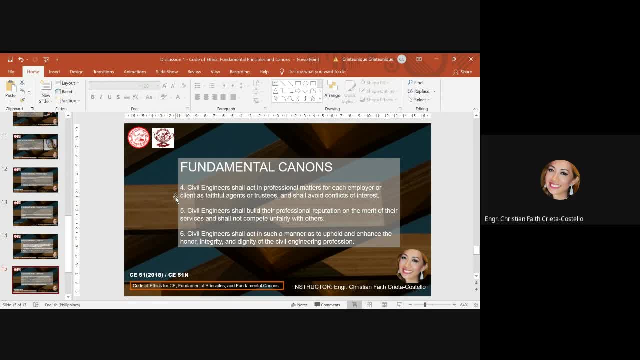 next number, four civil engineers shall act in professional matters for each employer or client as faithful agents or trustees and shall avoid conflicts of interest. yes, it is very common also and um workplace wherein if there is a jealousy that will exist, then conflict of interest will really happen, or if there is a greed, that 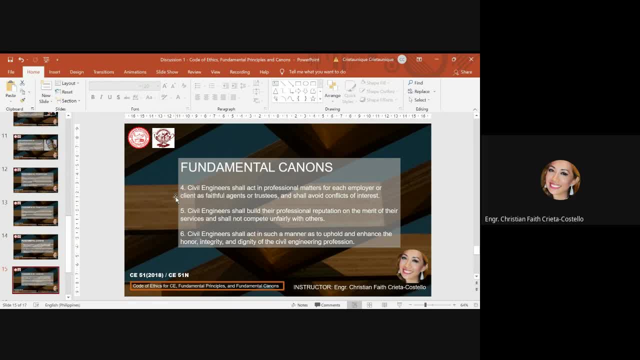 will exist. conflict of interest will really happen. so try to avoid feeling jealous or feeling greedy to whatever position or to whoever colleague and the company that you are working with, because it is very unethical and unprofessional. next is civil engineer shall build the professional reputation on the merit of their services. 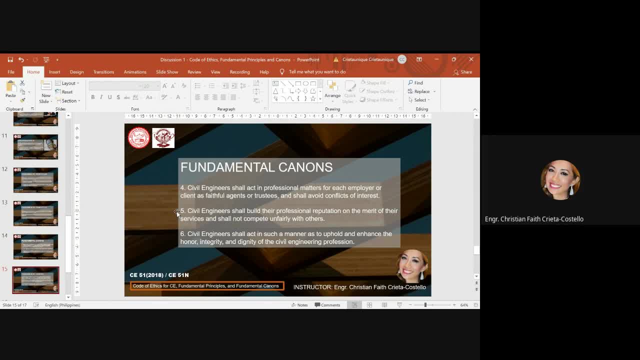 and shall not compete and fairly with others. yes, you should build your professional reputation by simply doing good work, but not that. never make your like, never make your background as a civil engineer very good by competing and fairly with others. or say by: I can give you a situation, say you want to make your civil engineering? 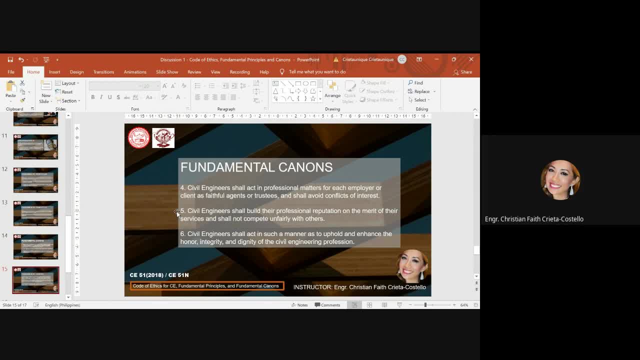 background or as a construction firm owner, you want to have your company background really look good. then as much as number of projects you want, then you want to list it down but to to know in reality you are always like doing and fair practice of bidding wherein you tried to befriend or give money to the bidding official so that 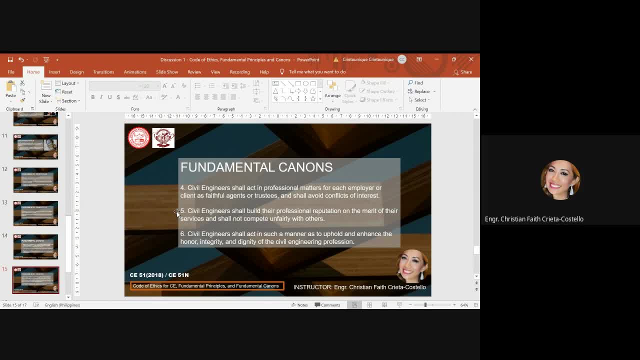 you will always win in every bidding situation, then this could be an example wherein a you are already getting merit or good reputation for your company. however, in reality, you are competing unfairly. Next is: civil engineer shall act in such a manner as to uphold and enhance the 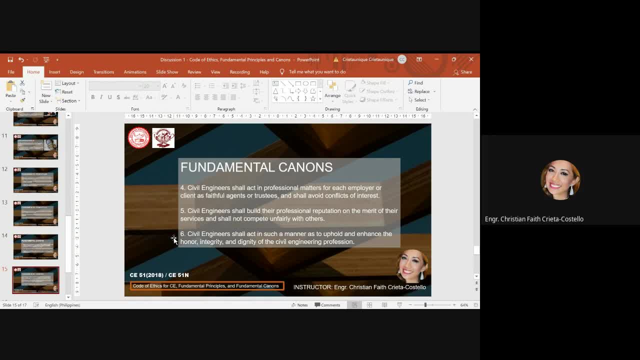 honor, integrity and dignity of the civil engineering profession. so this is always repeated: that we should always uphold and enhance the honor, integrity and dignity of the civil engineering profession. you should not forget this one, even as a student- and even you will become professional civil engineer soon- always uphold and enhance the honor, integrity and dignity of the civil 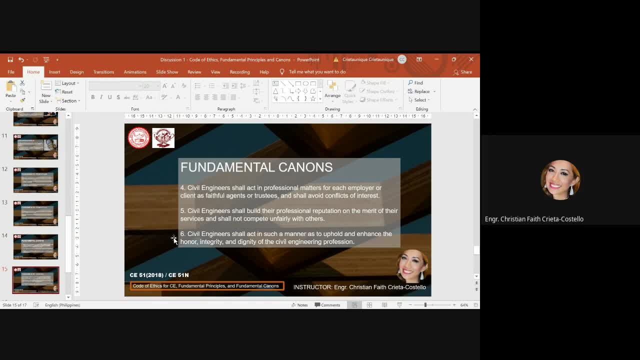 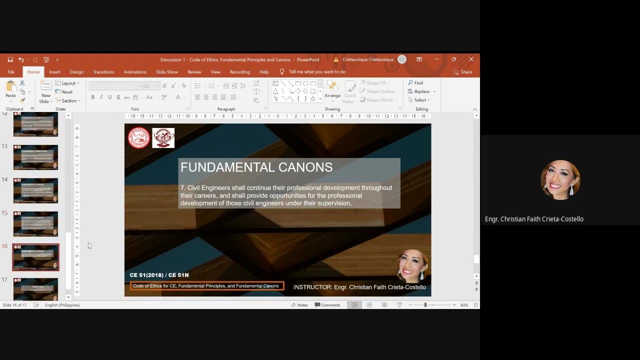 engineering profession because you have chosen this profession. therefore, practice the good ethics in this profession. then I think it is the last fundamental finance wherein civil engineers shall continue their professional development throughout their careers and shall provide opportunities for the professional development of those civil engineers and under their supervision. so to 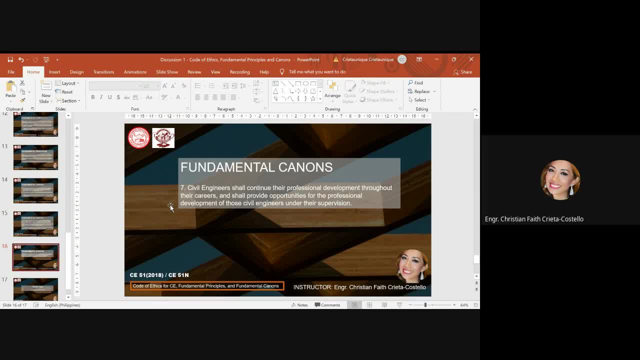 continue the professional development. sample of this is: it does not mean that you have graduated in civil engineering and passed the licensure exam, then you your civil engineering career will end there, or there could be way wherein you can still advance and develop your civil engineering. pursue like taking 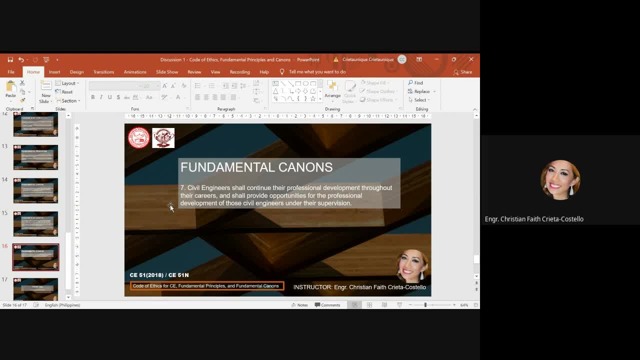 masters in civil engineering and then proceeding to a doctorate of civil engineering or, if not, simply trying to gain more knowledge on any other aspect related to civil engineering by simply doing your own research or even making research and make it published and do publications and also, at the same time, like sharing your knowledge to young civil engineers. 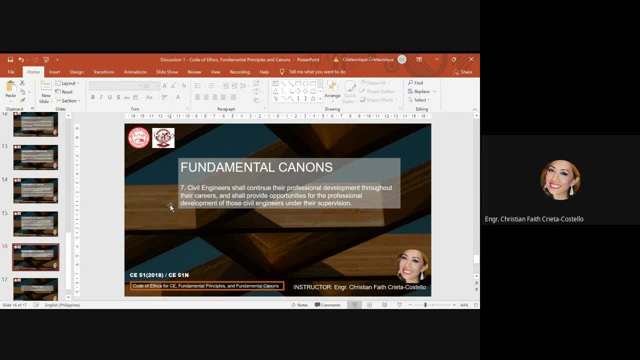 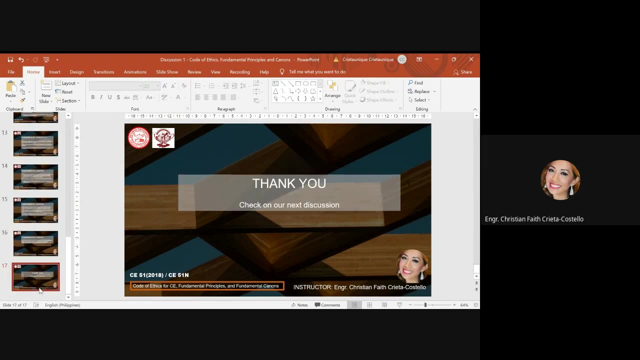 or even to students in civil engineering. so by doing this, you are performing the number seven, wherein you are continuing the professional development as a civil engineer. so this is what we have right now for code of ethics for civil engineering, fundamental principles and fundamental canons. I'd like you to check more on our next. 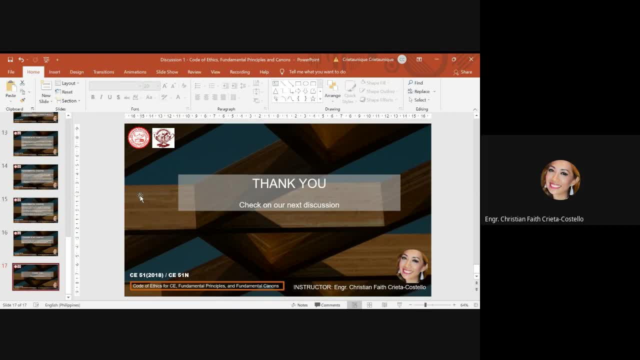 discussion related to civil engineering laws and ethics. thank you.